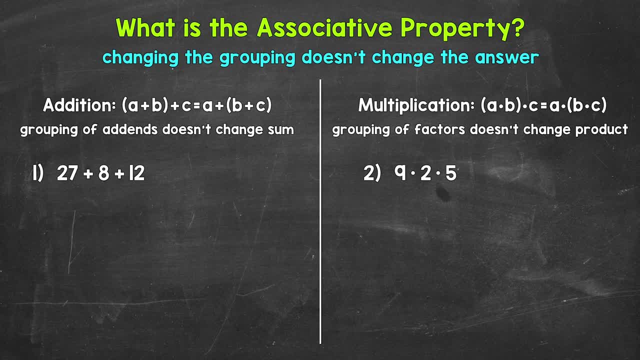 Let's take a look and use some numbers in order to see exactly what this means. For number one, we have 27 plus 8 plus 12.. Now let's start by grouping 27 and 8 and add these numbers. So we have 27 plus 8, grouped plus 12.. 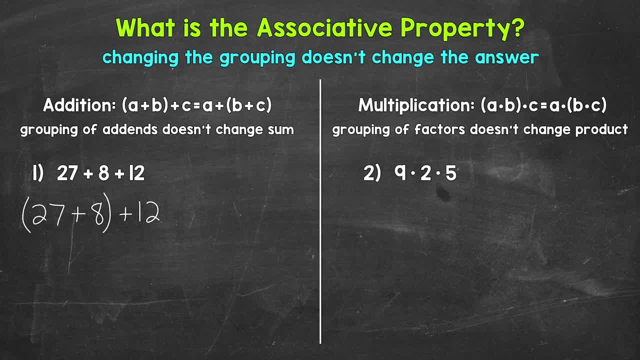 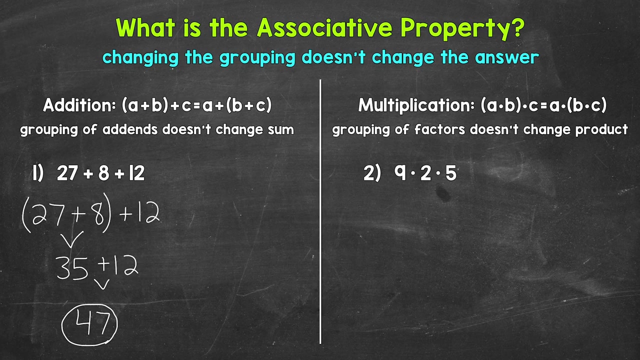 Now we can add, starting with the parentheses, 27 plus 8, that equals 35. Bring down the addition sign and the 12. We end with 35 plus 12,, that equals 47. Now let's group the 8 and the 12 and see if we get the same thing. 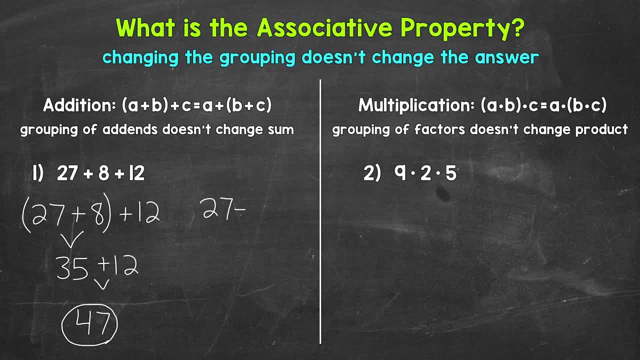 So we have 27 plus 8 plus 12 grouped. Let's add the 8 and the 12 and see if we get the same thing. So we have 27 plus 8 plus 12 grouped. Let's add, starting with the parentheses. 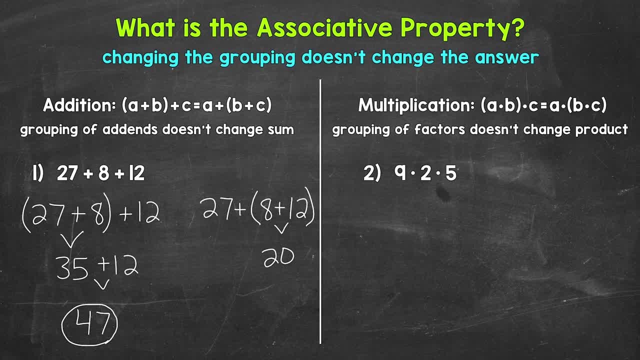 8 plus 12, that equals 20.. Bring down the addition sign and the 27. We end with 27 plus 20, and that equals 47 as well. So you can see that the grouping of addends didn't matter. 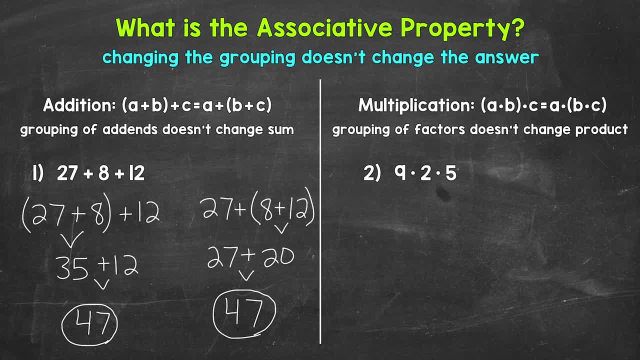 We got the same sum, the same answer either way: 27 plus 8, grouped plus 12.. So we have 27 plus 8 plus 12, that equals the same exact thing as 27 plus 8 plus 12 grouped. 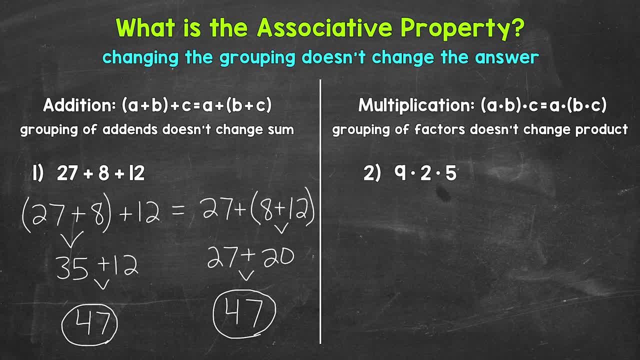 And that's the associative property. Let's move on to number 2 and take a look at the associative property of multiplication. So A times B grouped times C will equal the same exact thing as A times B times C grouped. The grouping of factors. 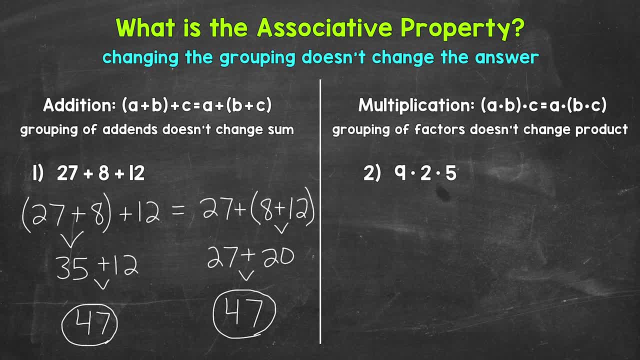 The grouping of factors doesn't change the product. Factors are the numbers being multiplied and then the product is the answer to a multiplication problem. Let's take a look at the example where we have 9 times 2 times 5.. Let's start by grouping 9 and 2..